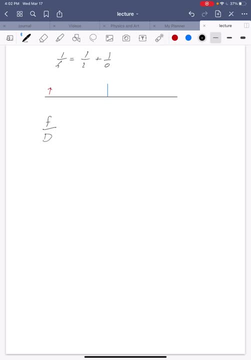 light to be able to take the picture, and oftentimes when I have a camera, the big pieces of instrumentation that exist are around the lens, which is fixed, and then the f number and the exposure time. So what I need to make sure is that I have enough light that comes in to take that picture. So the first thing is the f number. 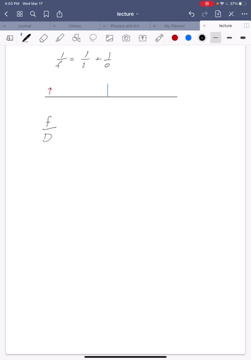 and the f number has to do with how much light is allowed in through the aperture, which is sort of a plate in front of the lens that will allow in different amounts of light, and f number is defined as the focal length divided by the diameter of the lens. and all of these values are going to be in meters. 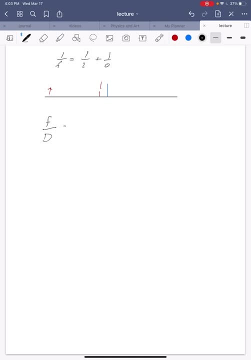 So when I do that, I end up with f numbers that are on the order of integer values, because the diameter of the opening is small compared to the focal length, f, And I end up with f numbers that look like, say, to four, uh and so on, and they don't actually double every time they go up by a factor of square root. 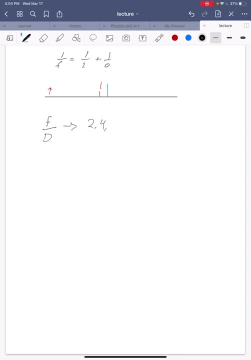 of two, because as i increase the radius, uh, what is important for the light is the area, and the area is pi r squared, so that's how you calculate f number. f number is also important because it determines the depth of field, which is a more complicated idea in photography. that, basically. 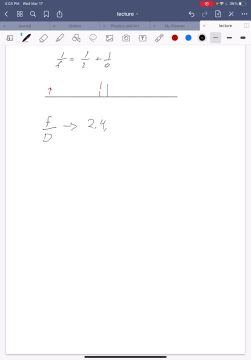 says that if i want to take a picture of the room and i want the whole room to be in focus, i need to be able to have images in the background be in focus enough and images in the foreground to be in focus enough that the picture as a whole looks uh, in focus. and to accomplish this we need to use 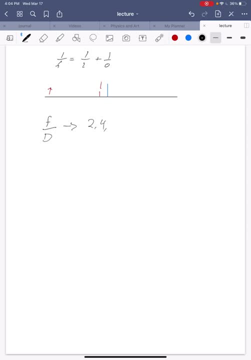 um, small f numbers, because this really lets the thin. uh, it minimizes the amount of light that we're going to be able to capture, and so that's why i'm saying that amount of bending from the edges of the lens. the other important piece of information is how long. 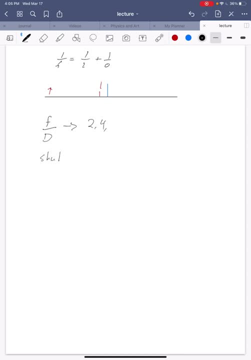 the shutter speed is. so the shutter speed has to do with how long this aperture is open and there are manual controls. but aside from that, usually we end up with something that are on the order of, say, half a second to. oftentimes it goes up to something like: 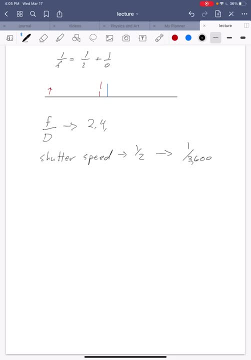 one three thousand six hundredth of a second. and if i'm taking a picture of a landscape, i can use this slow shutter speed, where if i'm taking a picture of a person running for, say, sports photography, i've got to use this high shutter speed because i don't want my picture to be blurry. so i have these two different aspects in play. 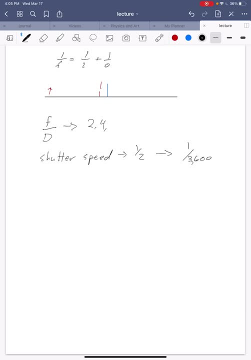 and i can get more light by by increasing the f number, which increases or decreases the f number increases the diameter, so that gives me less light. so as this goes up, i get less light, and as this goes up, i get more light. and for different applications, you want different. 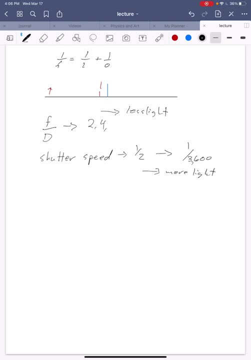 combinations of shutter speed and f number. so if i'm taking a landscape, i might use a very small f number to give me a very good field of depth and a very long shutter speed, because my landscape doesn't have a lot of motion, whereas when i'm talking about a 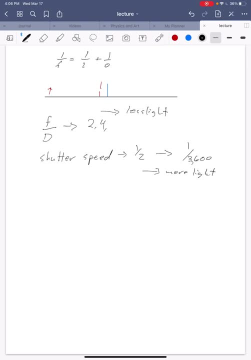 sports image. i'm going to use a larger f number and a shorter shutter speed so my image isn't blurry, but because of that the person or object i'm focusing on is in focus, but the foreground background aren't, and that gives us our picture of a camera. so again, the goal in big pictures. 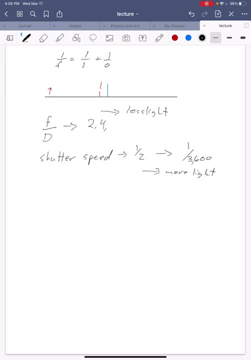 is to use the thin lens equation to understand where the object is or what focal length i need to achieve an image where the fixed photo player ccd is. and then beyond that i have these more complicated aspects of shutter speed and f number to determine the amount of light that comes in. so the smaller the f number, the less light. 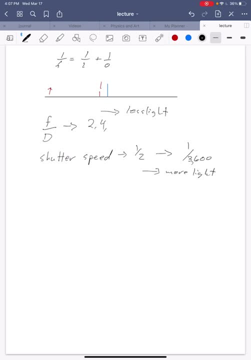 or the more light, but the worse. field of depth: the shorter the shutter speed, the more light, but the more likely it is for my image to become blurred.